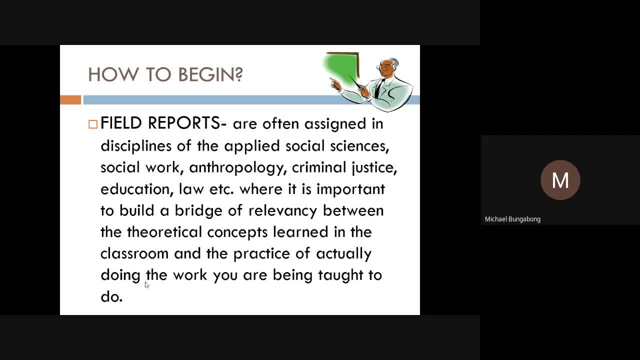 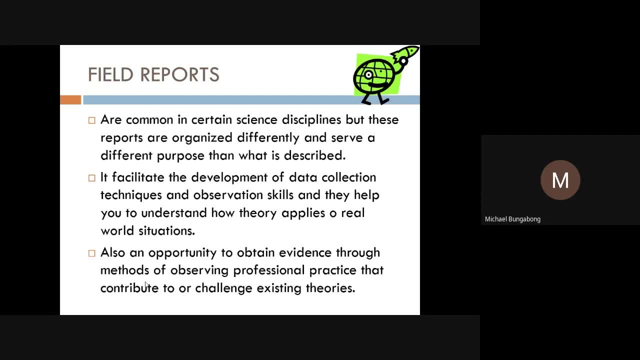 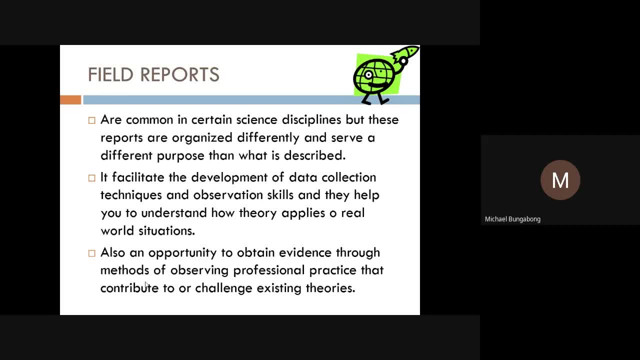 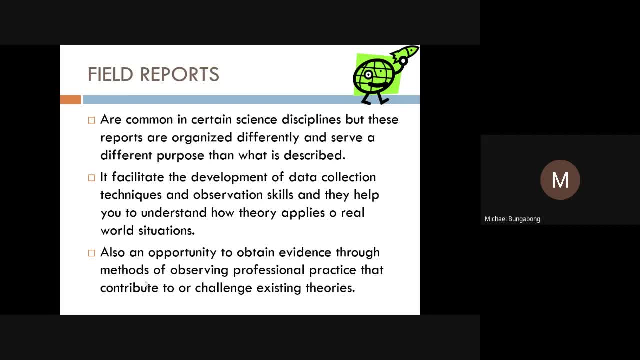 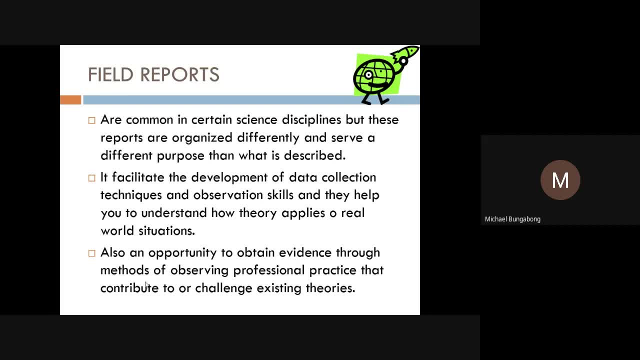 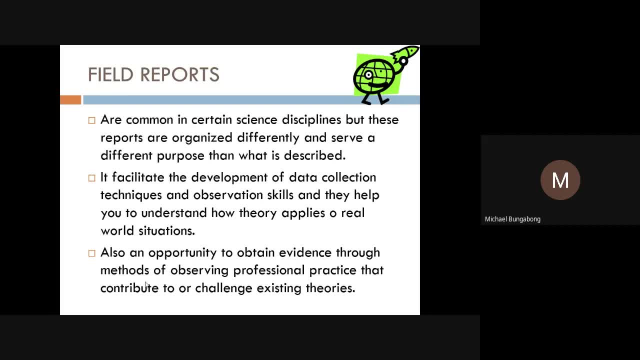 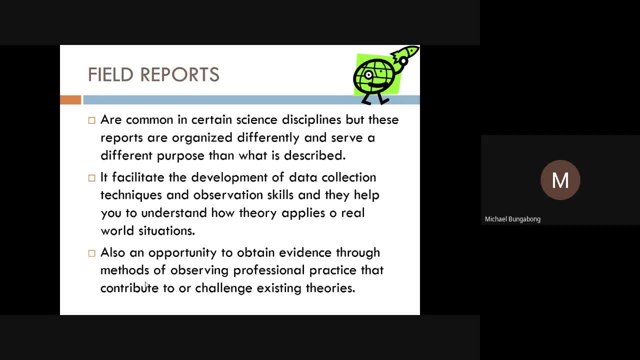 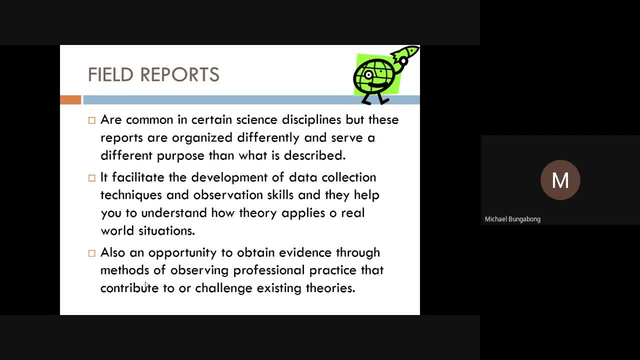 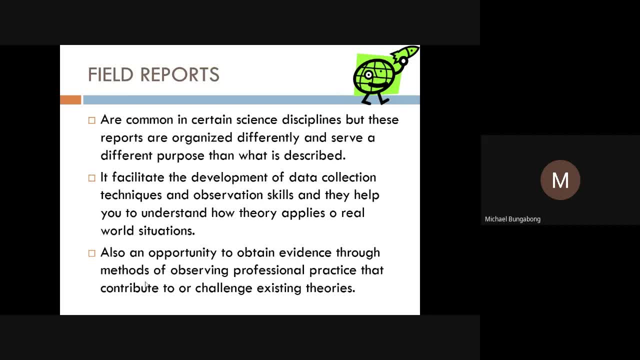 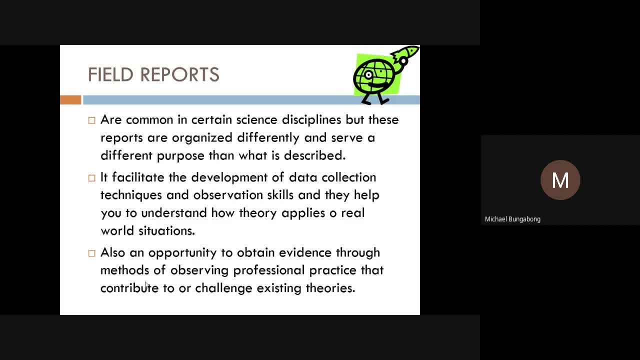 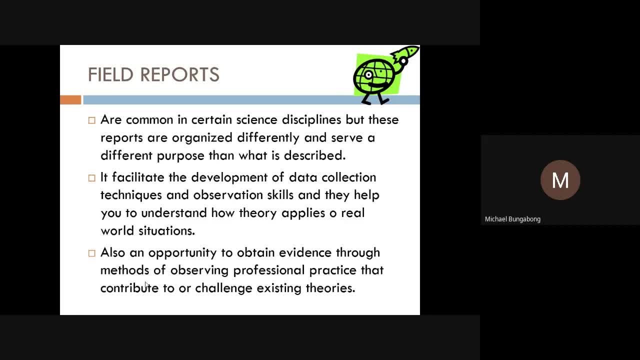 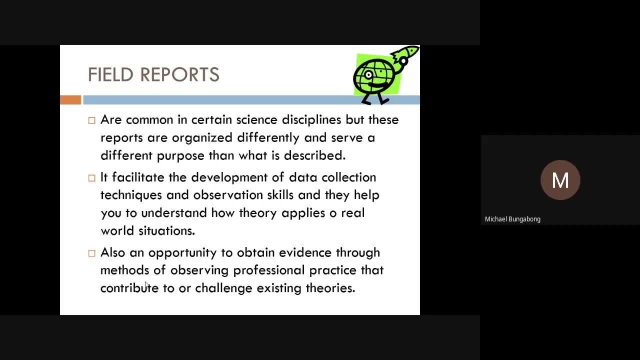 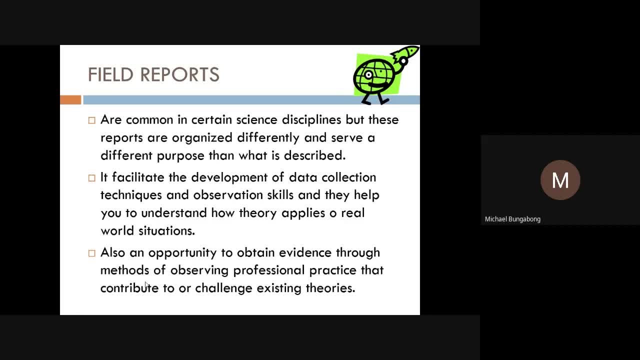 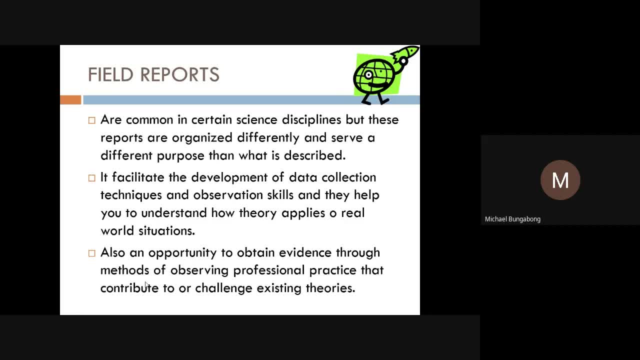 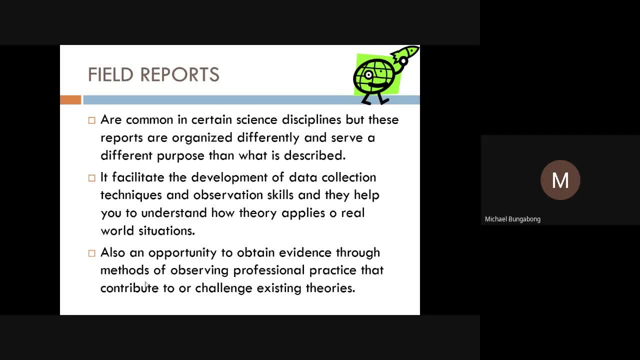 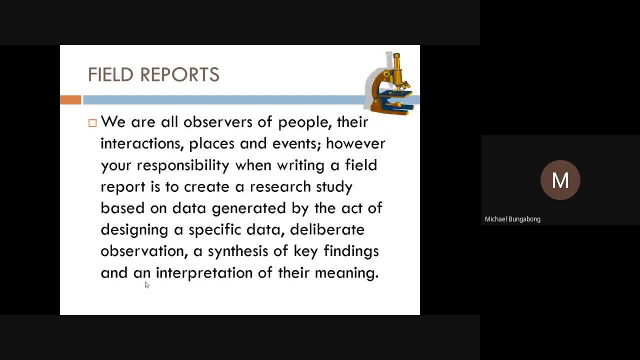 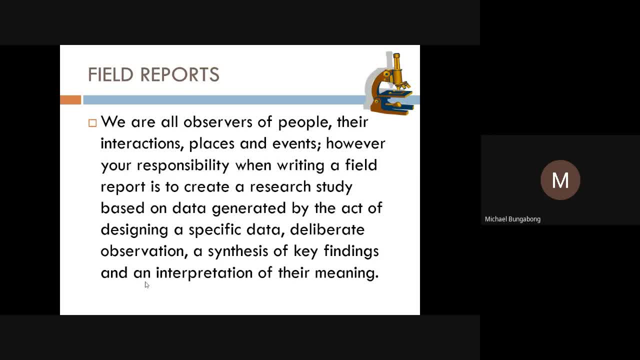 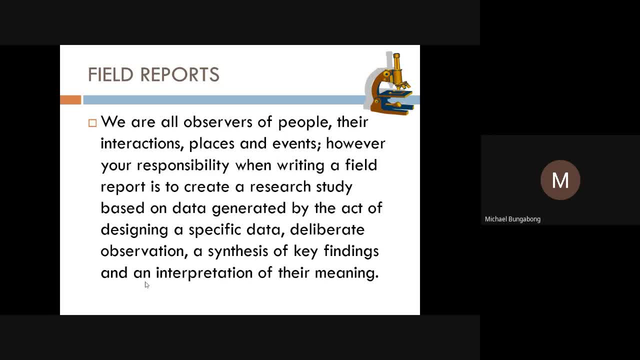 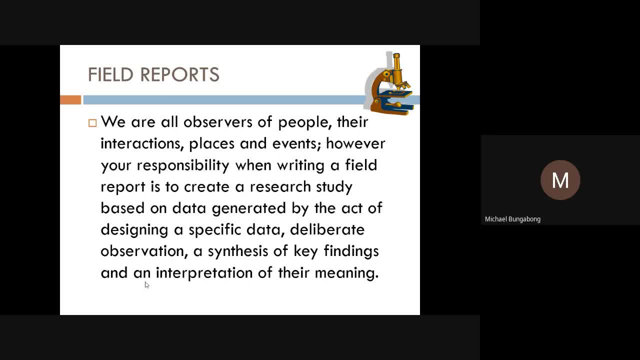 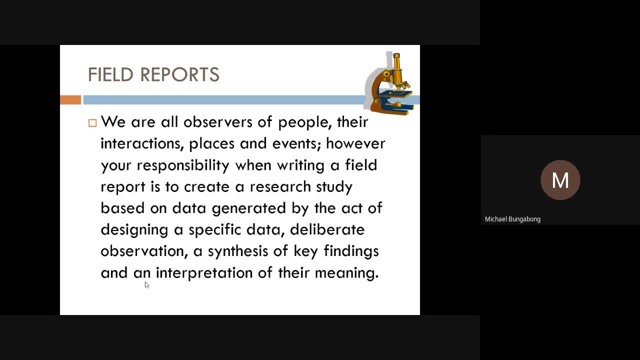 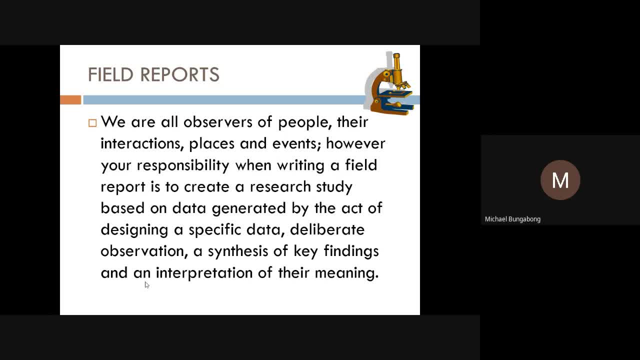 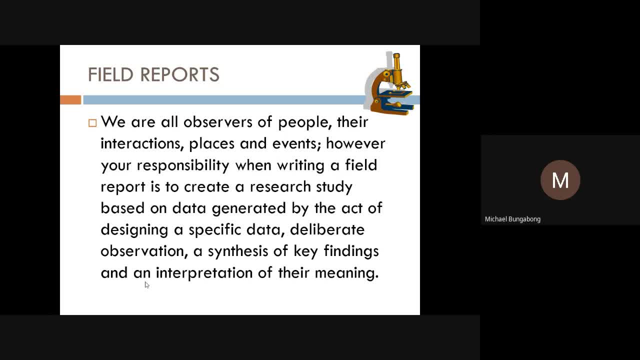 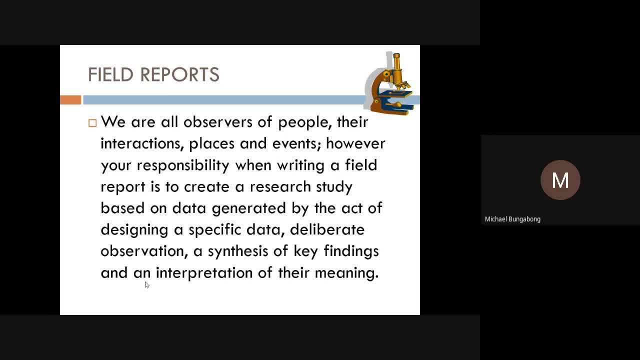 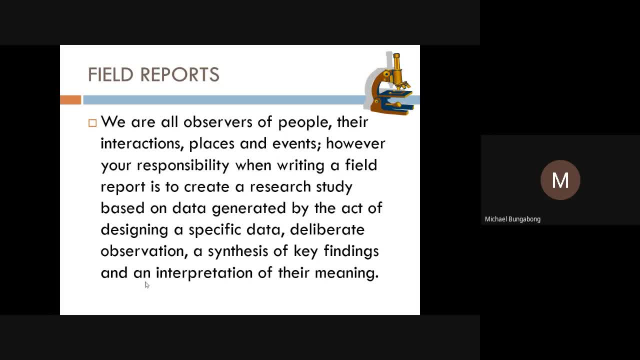 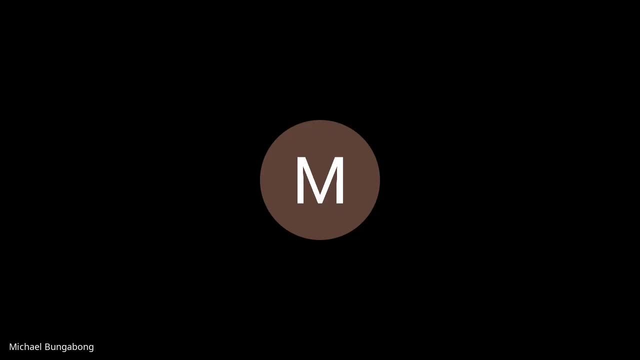 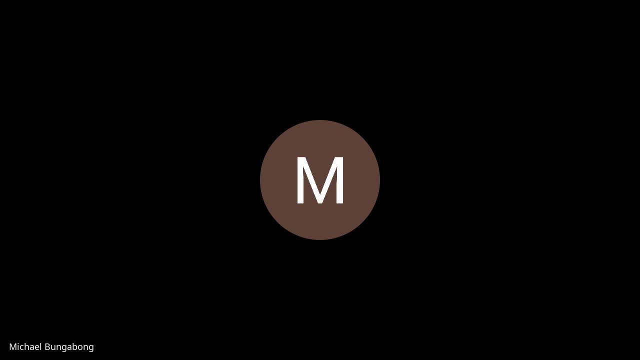 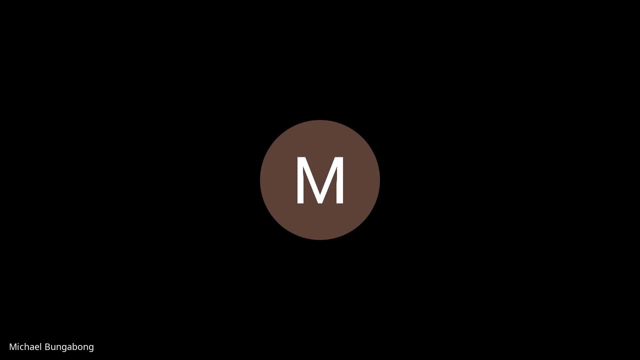 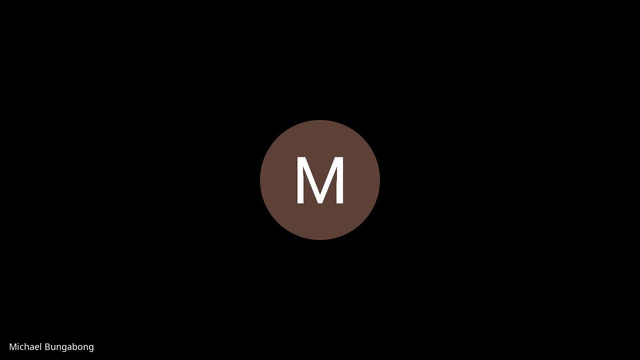 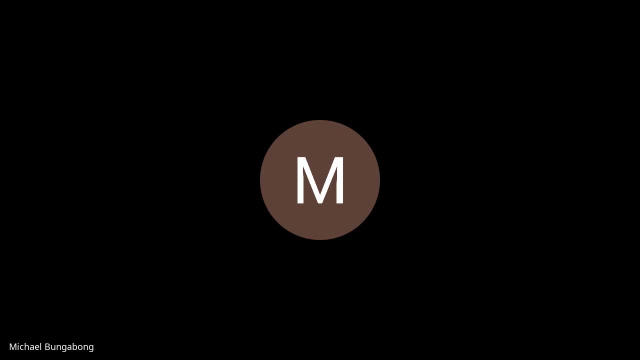 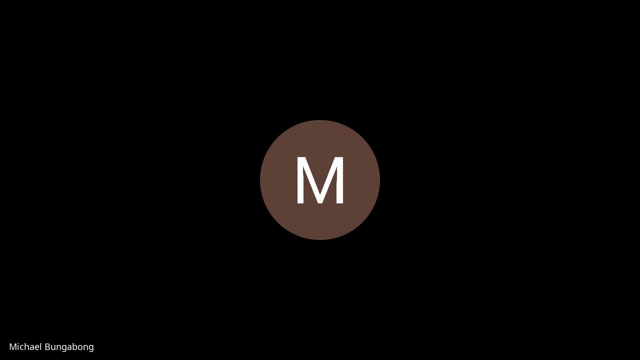 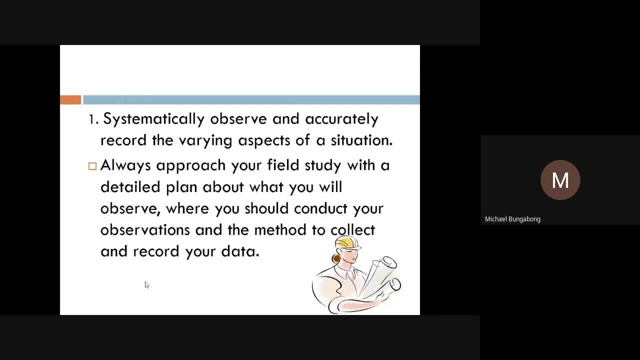 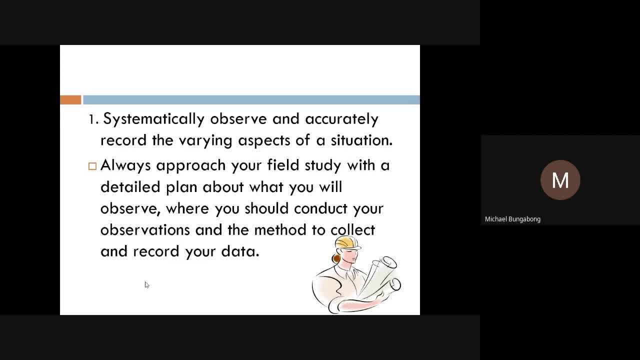 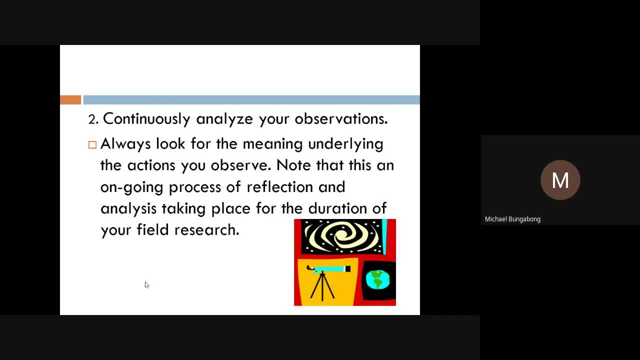 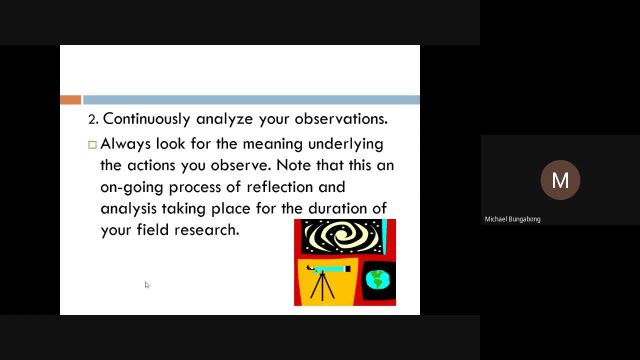 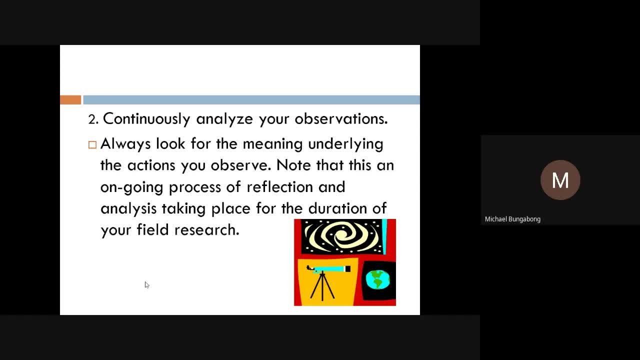 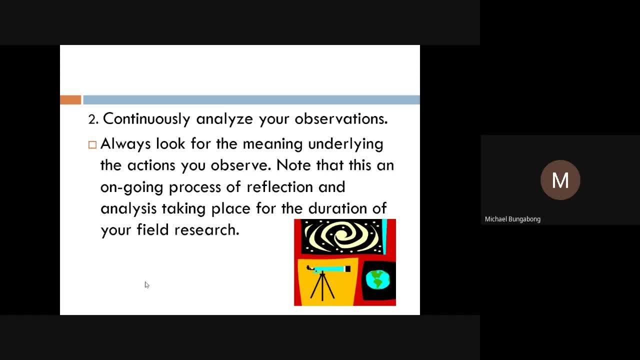 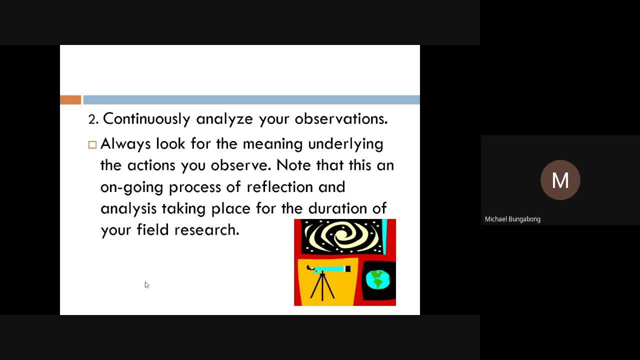 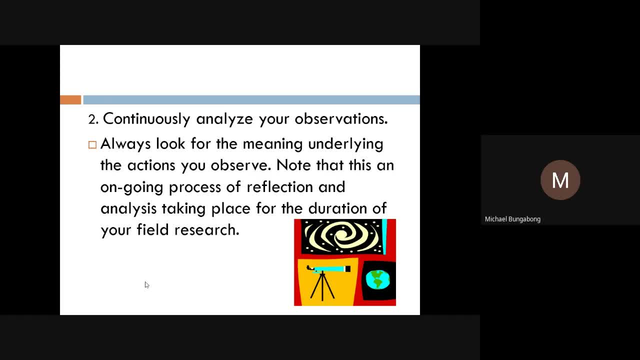 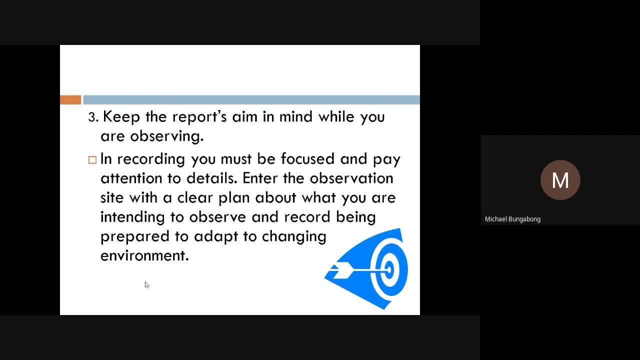 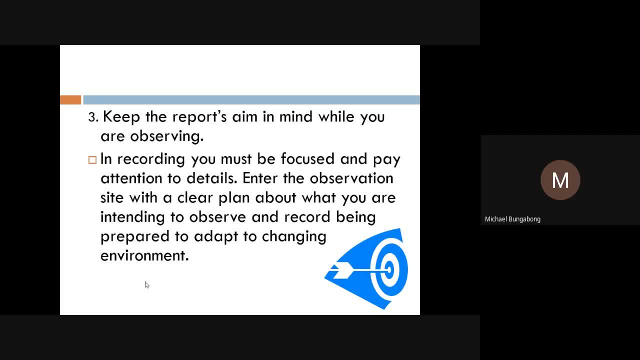 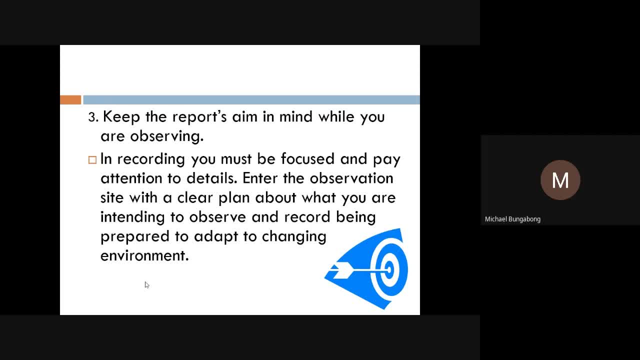 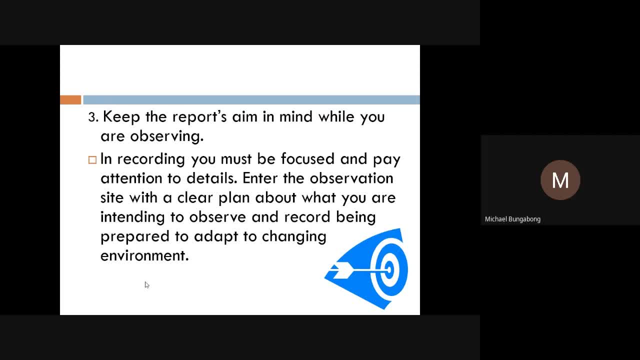 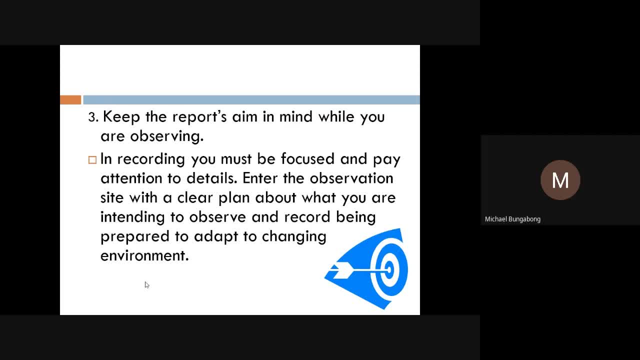 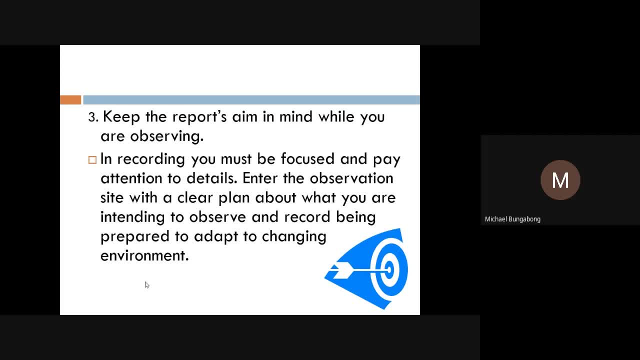 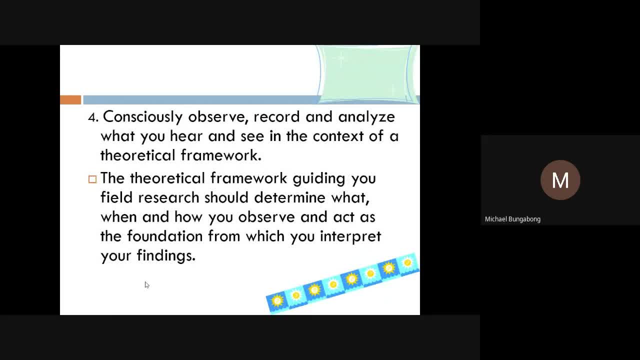 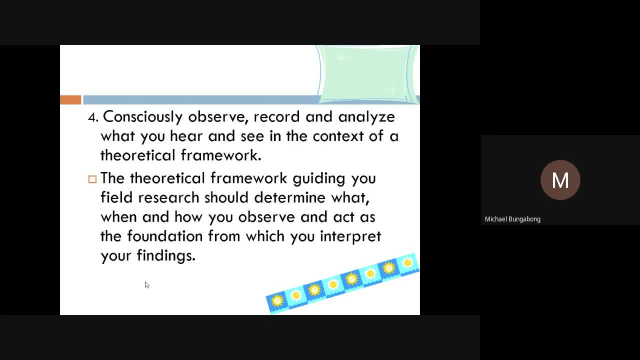 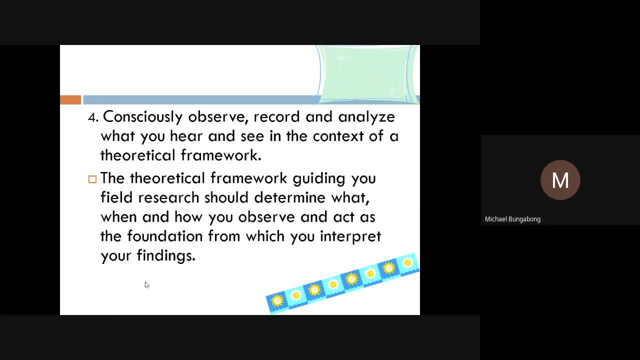 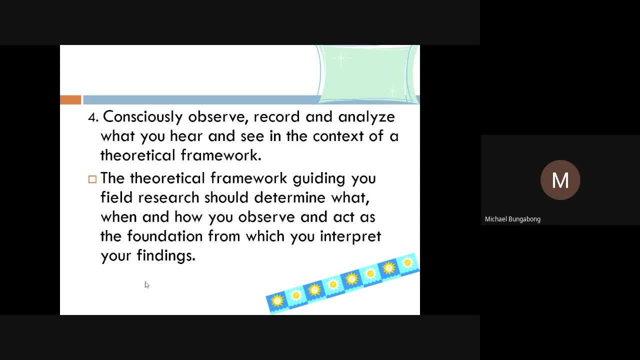 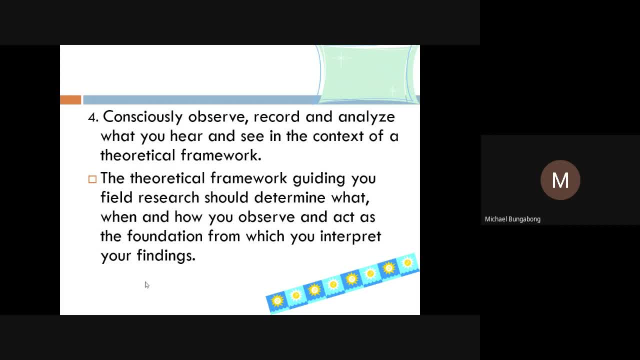 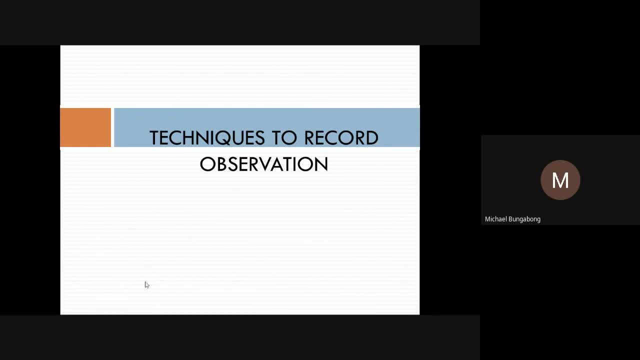 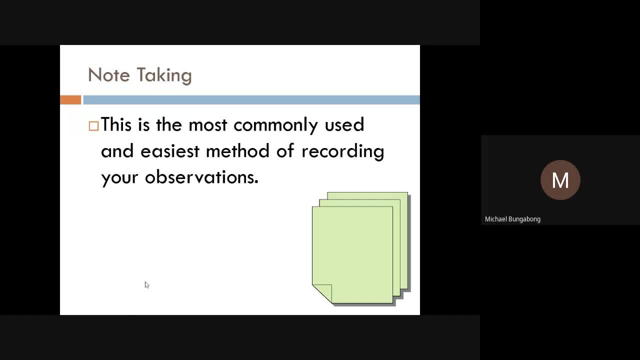 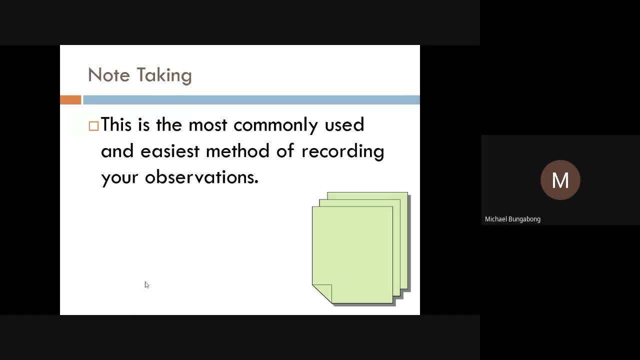 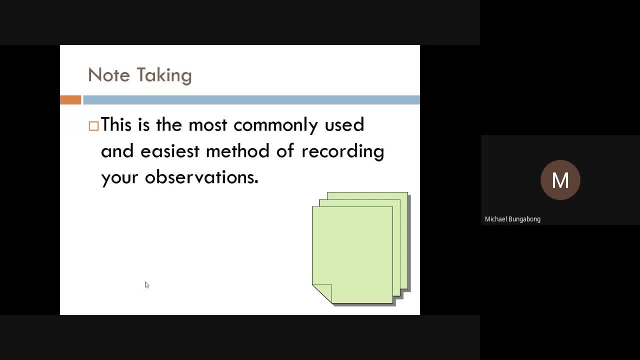 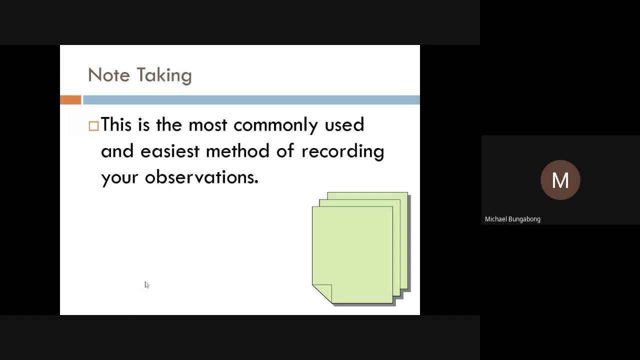 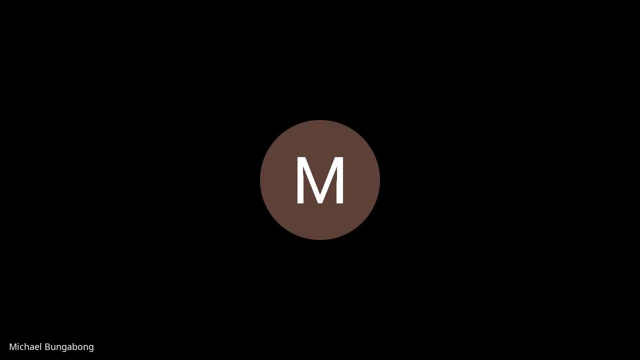 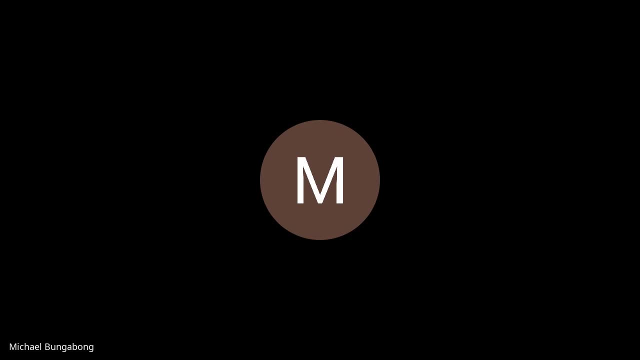 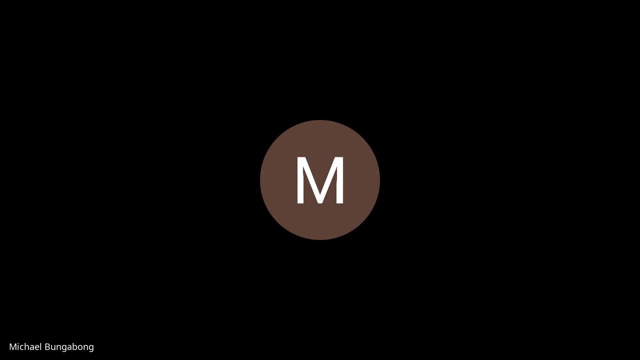 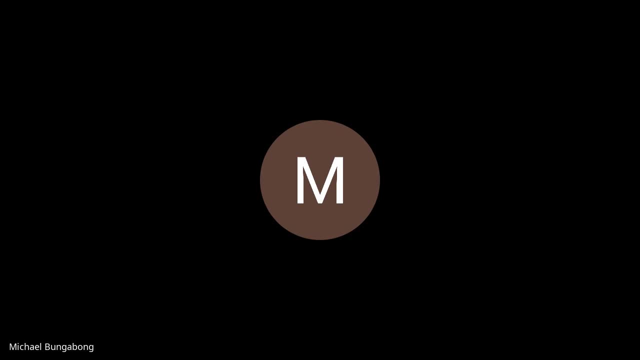 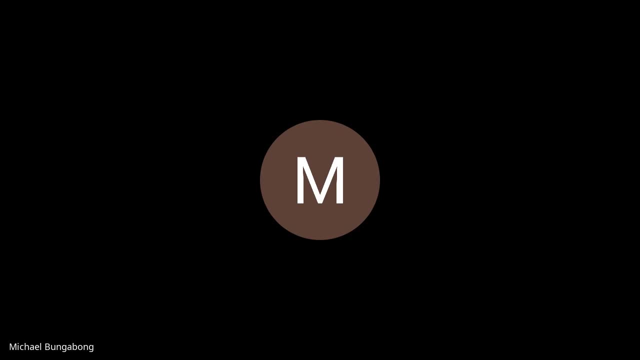 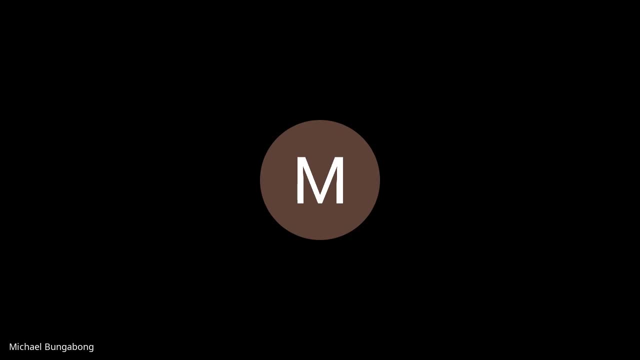 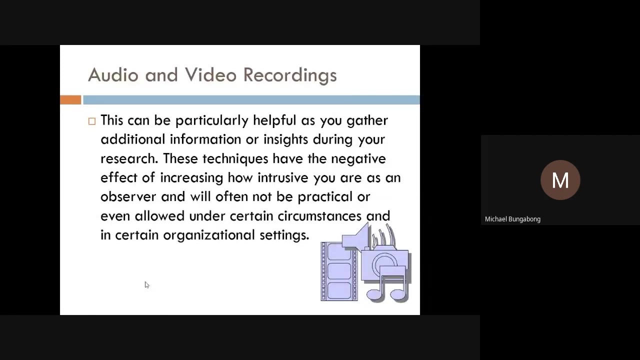 your writing. you know, and we also have the audio and video recording, so this can be particularly helpful as you gather additional information or insight during your research. so these techniques have the negative effect of increasing how intrusive you are as an observer and will often not be practical or even allowed under certain circumstances. 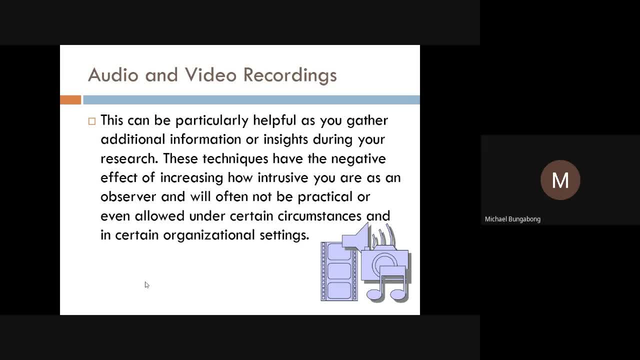 um, and in a certain organizational setting. so audio and video recordings is also vital when you do a field report, because in there you can uh have your own evidences, you have something to backtrack just in case that you miss something, and then you can cut the video. 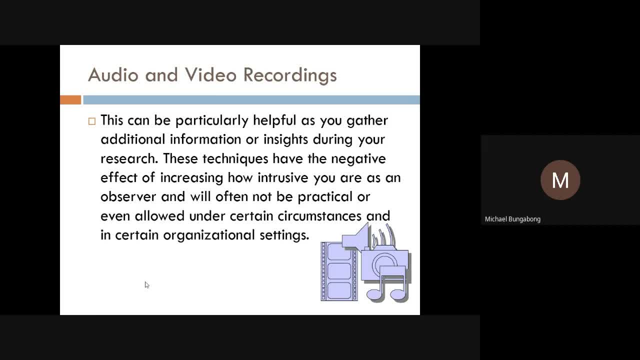 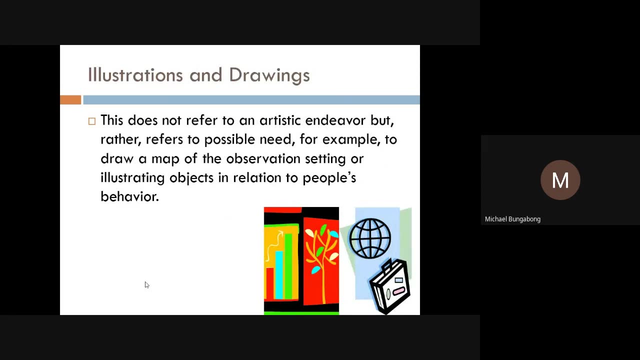 and go to the straight to the point. um, what are the, what are the relevance to justify your field works based on the recordings that you have? okay, then illustrations and drawings. so this does not refer to an artistic indie board, but rather refer to possible need, like, for example, to draw a map of the observation setting or illustrating objects in 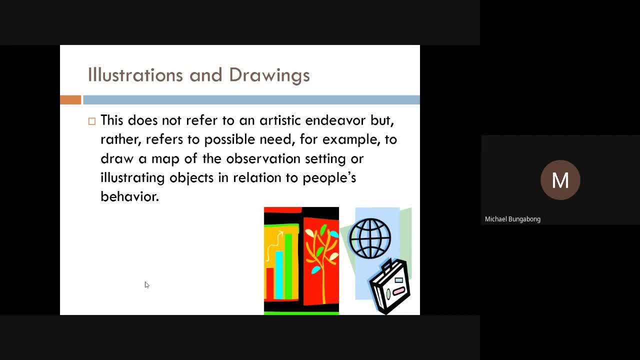 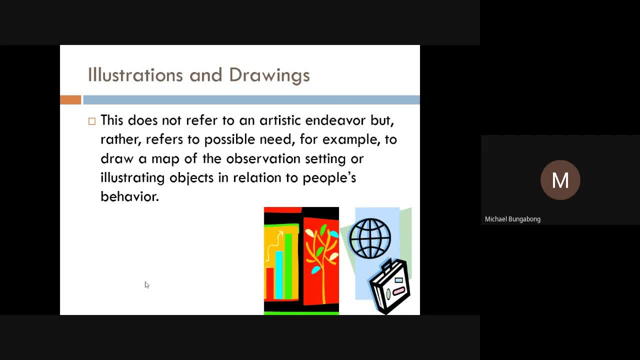 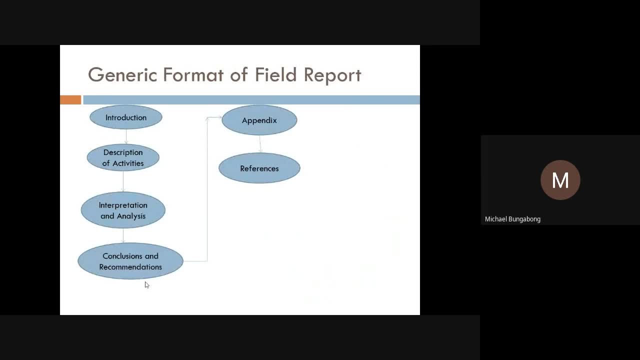 so definitely those illustrations and drawings will help your readers to guide them. okay, um, this is the generic format of field report. so we have introduction, then description of activities, interpretation and analysis, and the conclusion and recommendations and references. okay, so let's just discuss this generic format of field report one by one. 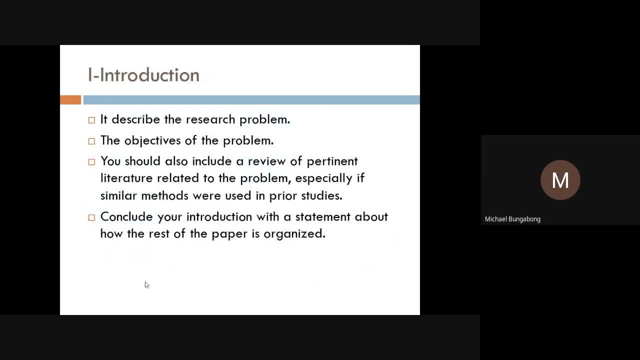 so in introduction class, it simply describes the research problem. okay, and what are your objectives? you should also include a review of pertinent literature, then conclude your introduction with a statement about how the rest of the paper is being organized. so that's- uh, these are the elements, or these are the important elements, of the report. so let's just take a look at the report one by one. 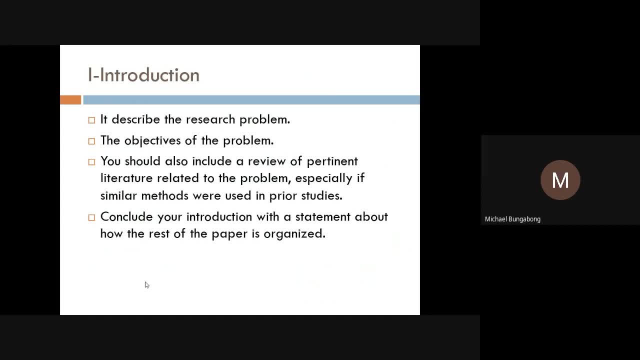 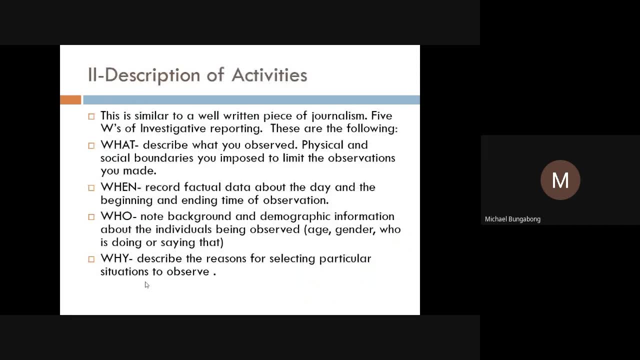 factor that we can see on your introductions. okay, and of course, let's go to the description of activities. this is similar to a written piece of journalism, like asking the 4w and each question like what, when, who, why for you to be able to figure your field report. okay. 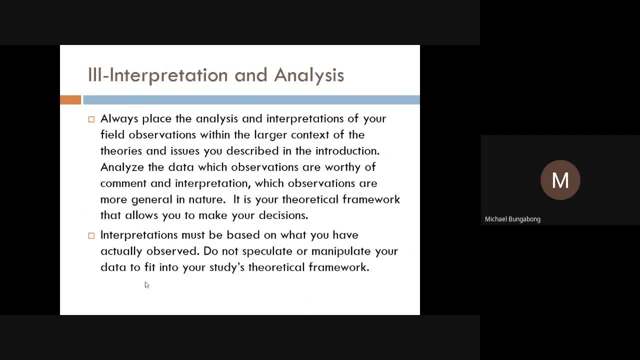 interpretation and analysis. classes always place the analysis and interpretations of your field observations within the larger context of the theories and issues you describe in the introduction. why is it? why is it so? because classes analyze the data, which observations are worthy of the comment and interpretation, which observations are more generated in nature. and it is your. 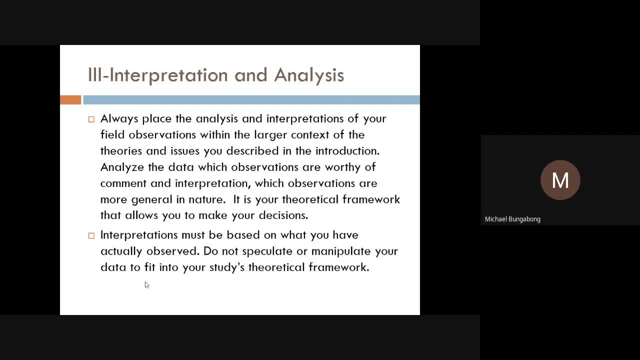 theoretical framework that allows you to analyze the data and interpret it in a way that is allows you to make your decisions. and, of course, it's also interpret. uh, i'm sorry. interpretation must be based on what you have actually observed. do not speculate or manipulate your data to fit. 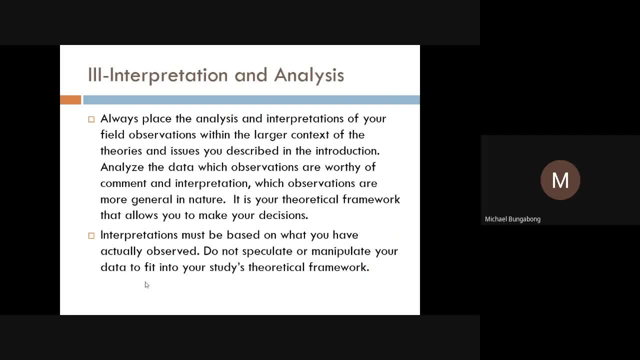 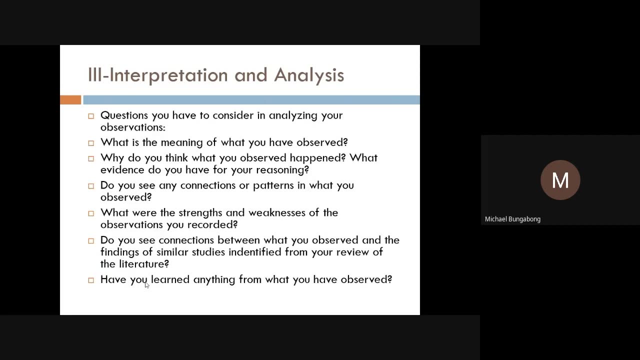 into your studies theoretical framework. so this is what i'm talking about: class. now you have to focus what is really happening based on what you see, what you observe. nothing more, nothing less. okay, so interpretation and analysis: these are the questions you have to consider in analyzing, or 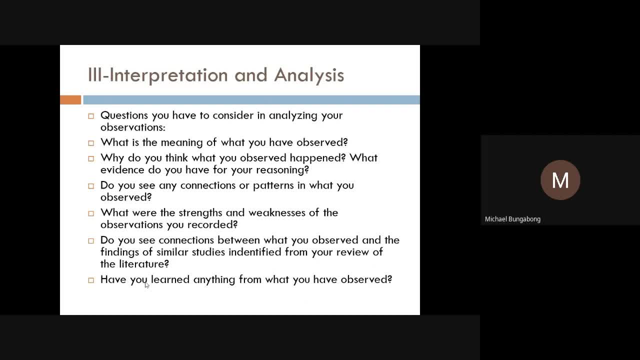 observation like: what is the meaning of what you observe? why do you think what you observe? do you see any connection or patterns? what you observe? what are the strength and weaknesses of the observations you recorded? do you see connections between what you observe and the findings? so these are the questions that will definitely help you out to shape your field report. 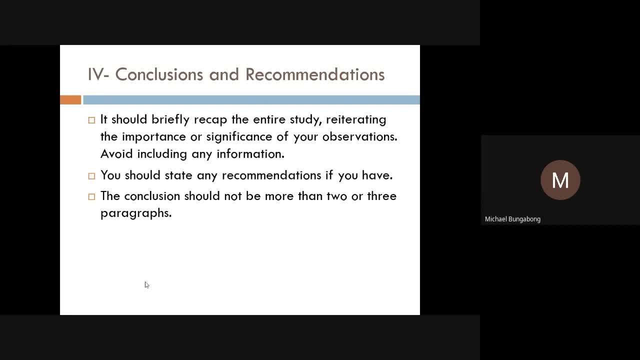 so of course we have conclusions and recommendations. it shows briefly recap the entire study, reiterating the importance of significance of your observations. avoid including any information, then you should state any recommendations, if you have, and then conclusions should not be more than two or three paragraphs, so the shorter the better. on the conclusions and 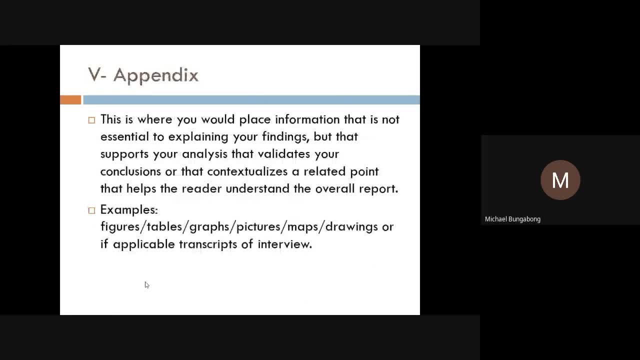 recommendations- if you have any recommendations- and, of course, appendix. this is where you would place information that is not essential to explaining your findings but that support your analysis, that validates your conclusions or that contextualizes or related point that helps the reader understand the overall report, like, for example, figures, tables, grab pictures, maps, drawings. 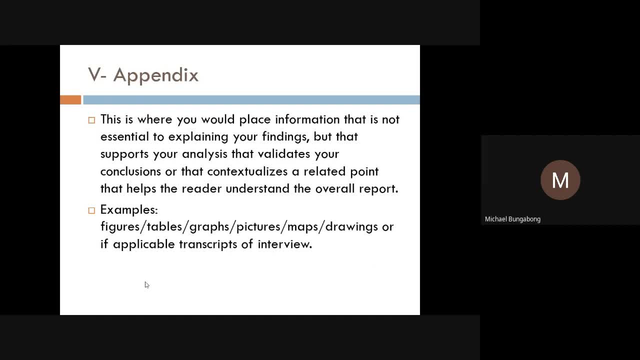 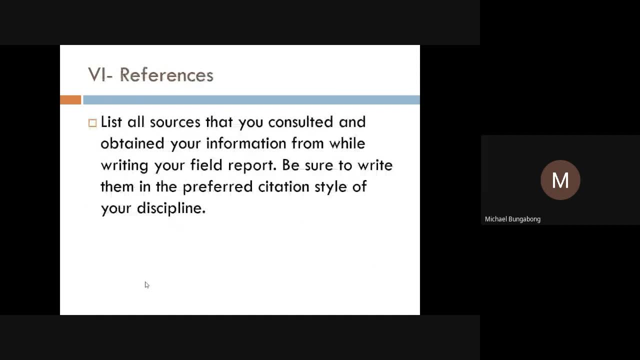 it will help your readers or your audience to understand it clearly what you meant to your uh, to your field report and, of course, references. so these are the least all sources that you consulted entertain your informations from well from while writing your field reports. be sure to write them. 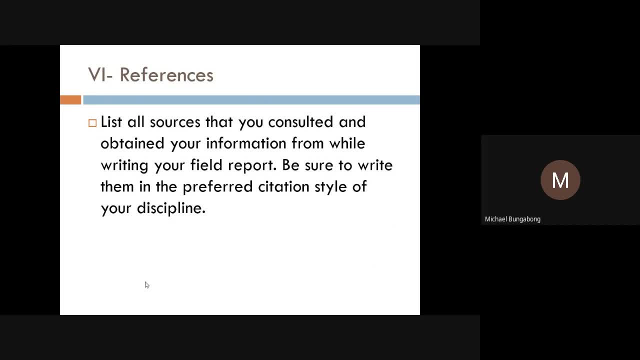 in the prepared citation style of your discipline. so it depends what are the type of citation that you want to like um on, if that is online, if that is from the book, and it's all up to you. uh, well, we are not going to go into that, but, uh, as of the moment, um, we're done discussing that, but of course, 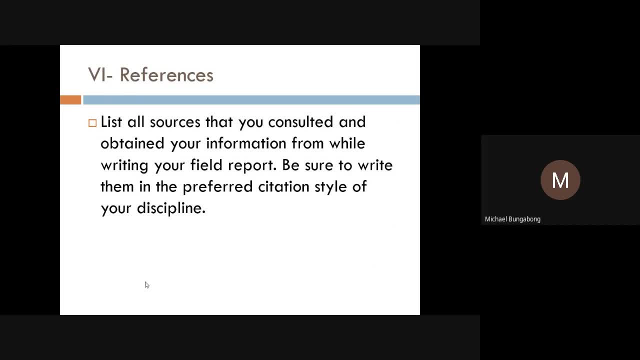 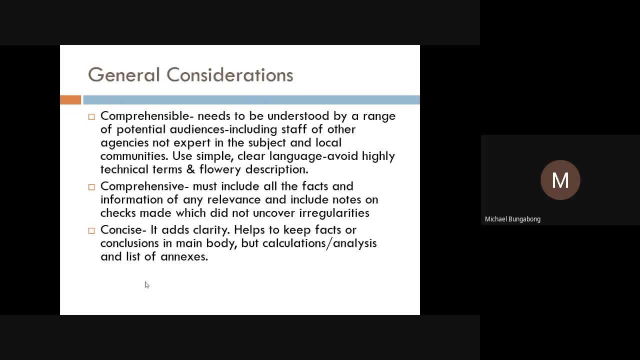 we're not going to go in there, so i hope that you know how to do e, uh, to write e, certain references okay, and, of course, general considerations. we have the three c's that we have to consider like comprehensible: what, what, com, friends, what comprehensible means? uh, it needs to be.